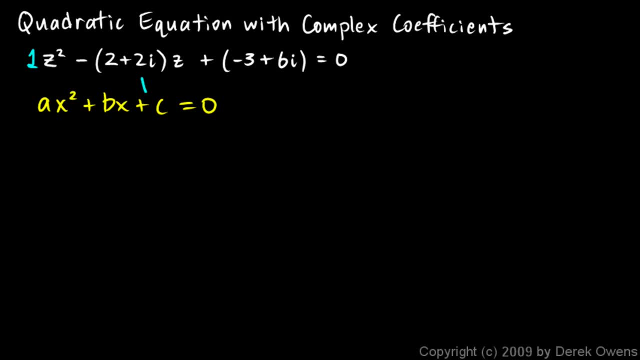 right there with a little line through them, just so they're not mistaken for a 2. okay, the quadratic equation you probably remember can be solved with the quadratic formula. any equation in this form can be solved like this: x is negative, b plus or minus, the square root of b squared minus 4ac. 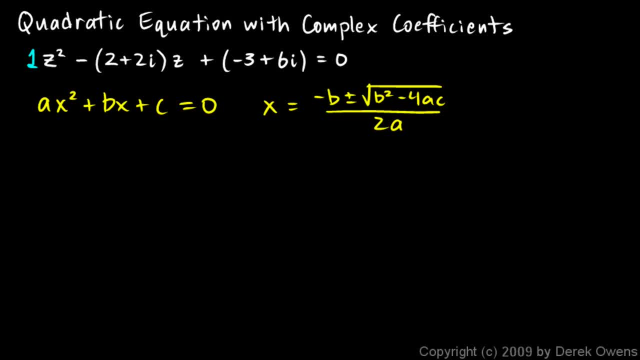 all over 2a. well, the same formula applies here, we just have some complex numbers involved. this is a: a is equal to 1 and this is b: b is equal to negative 2 plus 2i, or you could write it as negative 2 minus. 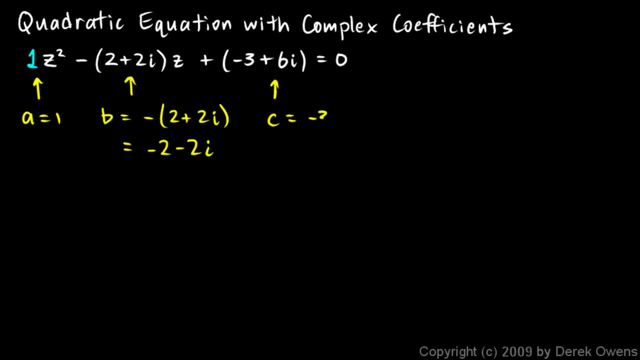 2i, and then this is c. c is equal to negative 3 plus 6i, and then z is going to be negative. b z, which is our answer, is going to be negative. b plus or minus. the square root of b squared minus 4ac. 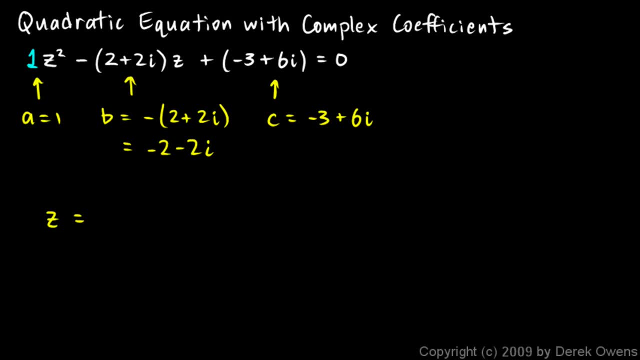 all over 2a. so let's write that negative b is just going to be the opposite this, so it's going to be 2 plus 2i, plus or minus the square root of b squared, so b is: is this negative 2 minus 2i? 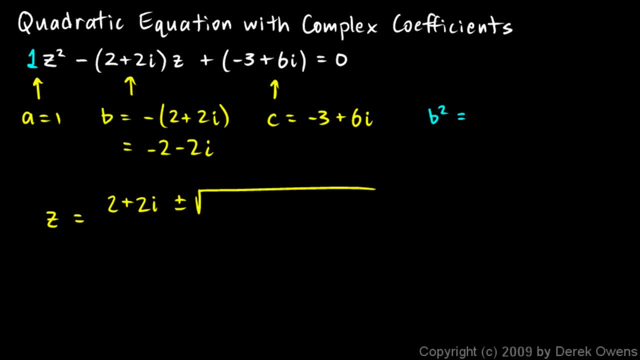 so let's figure out what b squared is going to be. b squared is going to be negative 2 minus 2i squared, so you can work out a foil. here you get a 4. let's see plus 4i, plus 4i, plus 4i squared and the 4i squared- i squared, remember- is negative 1. 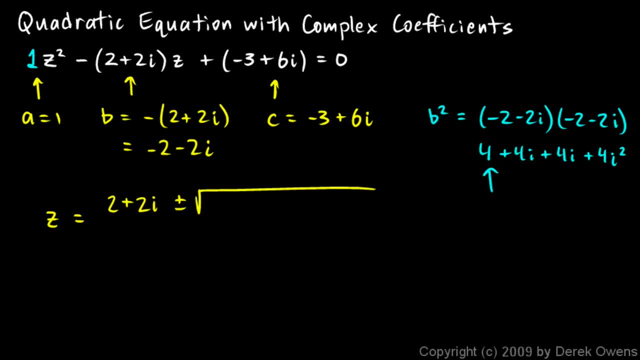 so this is a negative 4 and that's going to cancel out with this 4 here. so b squared is just equal to 8i. so in our radical here we have a 8i, that's b squared minus 4 times a, times c and all that's. 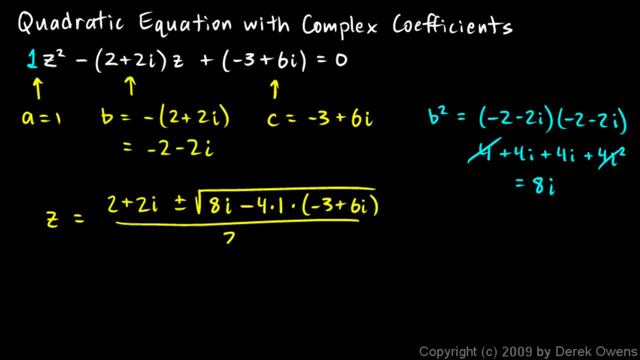 over 2a and a is just 1, so 2a is just going to be 2. so now let's work this out and see if we can get an answer. z is going to equal 2 plus 2i, plus or minus the square root. 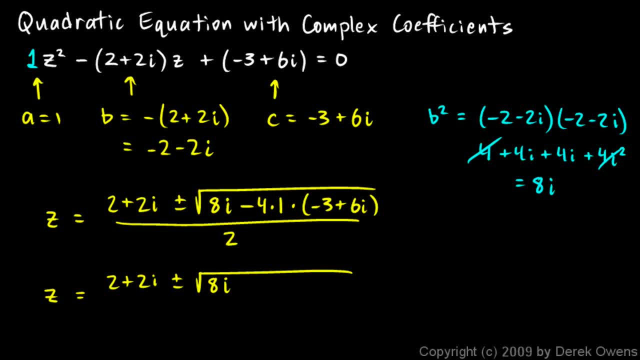 of this is 8i, and now let's distribute this 4. we have a minus 4 right here times a negative 3, so that's going to give us a plus 12. and then we have a minus 4 times a plus 6i, so that's going to give us a. 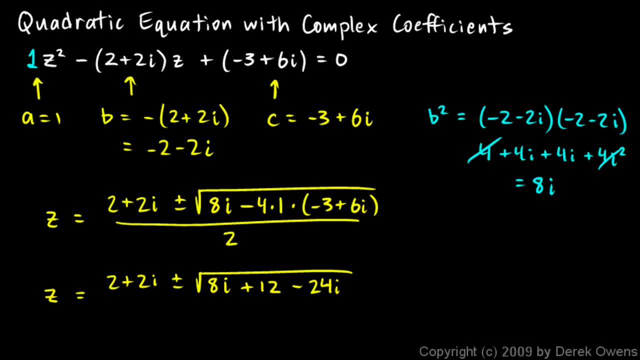 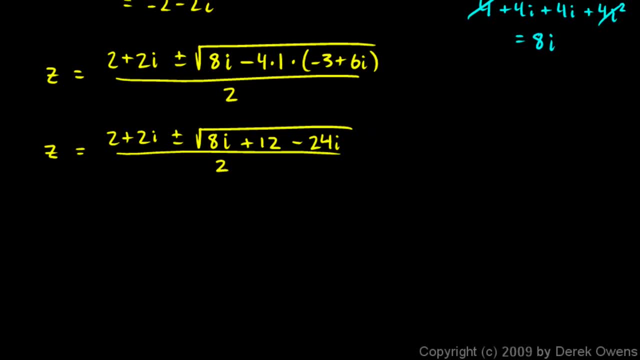 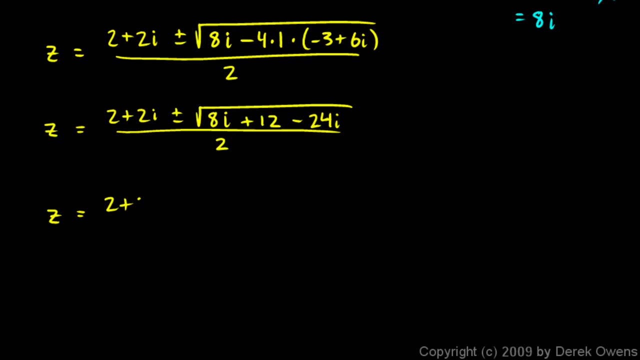 minus 24i and all that's divided by 2. I'm going to scroll down a little and continue here. z will equal 2 plus 2i, plus or minus the square root. I'm just going to combine like terms up here. that's a 8i and a negative 24i is going. 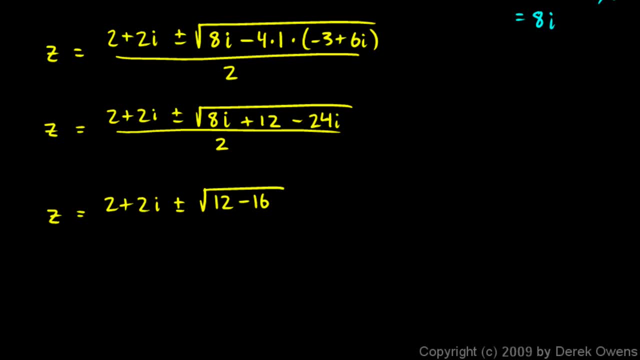 to give me up minus 16 i. so this is a 12 minus 16 i under the radical, and we can simplify this a little bit, and simplifying it always helps, so let's keep this 2 plus 2i out here for a second. 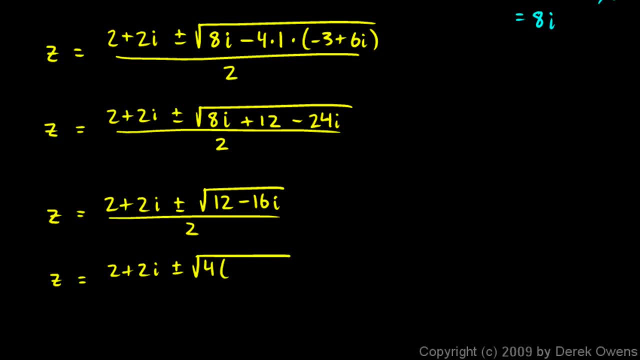 under the radical. I can factor out a 4 and that leaves me with a 3 minus 4i over 2, and then you can see the 2's cancel. actually, right here let's rewrite: that is 2 times 1 plus i. I'll go ahead and show this next intermediate step where the 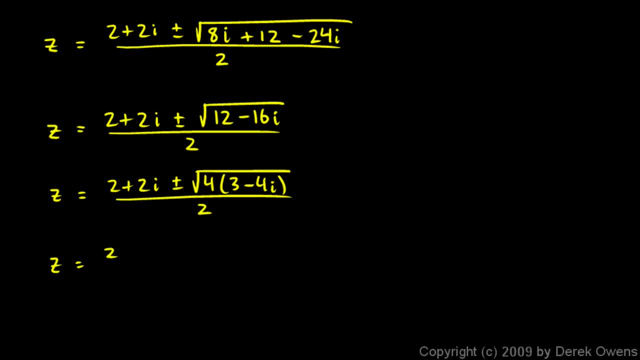 2's appear. before I cancel them, Let's write this as 2 times 1 plus i. This 4 under the radical will pop out as a 2, so I have plus or minus 2 times the square root of 3 minus 4i. 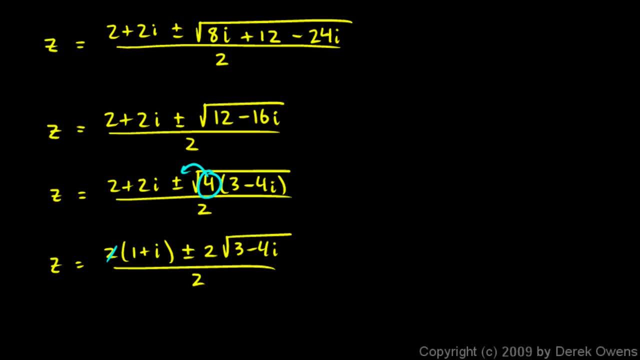 a 2 on the bottom and then you see all these 2's canceling, so that makes it a little simpler. so then I have: z is just 1 plus i plus or minus the square root of 3 minus 4i. Now what is this? 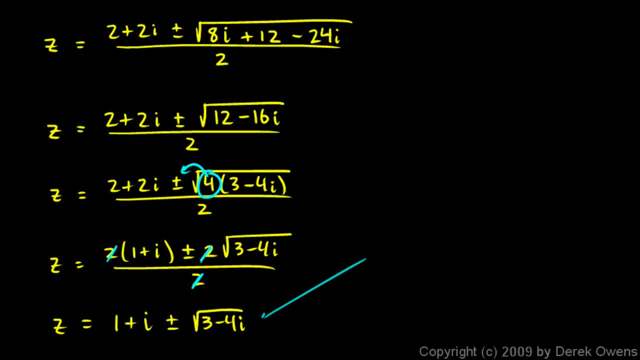 the square root of 3 minus 4i. I'm going to go ahead and tell you that the square root of 3 minus 4i is equal to 2 minus i, and I'll come back at the end and elaborate on that. but let 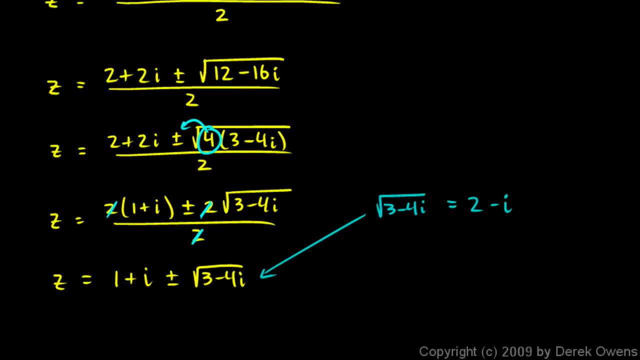 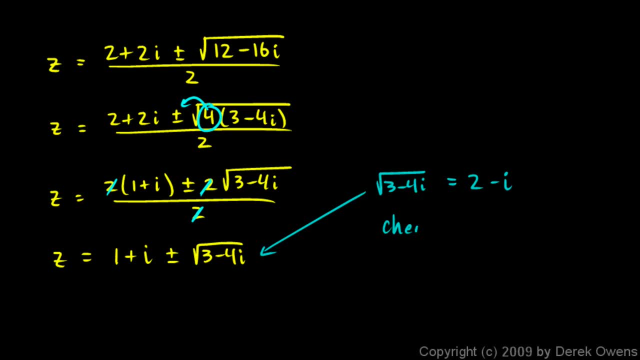 me just prove to you that that is the case. Watch this: if I take 2 minus i and square it, I should get 3 minus 4i. so let's just check that real quick: 2 minus i, squared, 2 minus i, times 2 minus i, That's going to equal doing a. 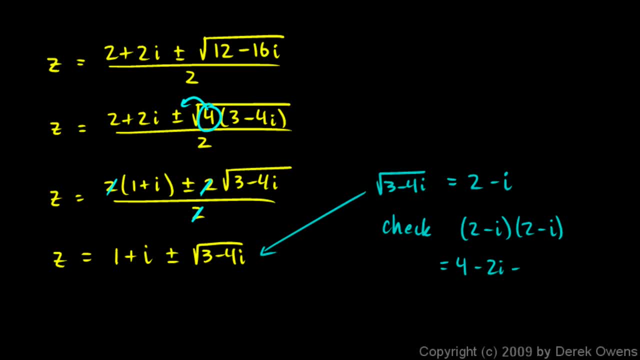 FOIL here: 4 minus 2i minus 2i plus i squared, and i squared is negative 1, so this is 4 minus 4i minus 1, which is 3 minus 4i is 3 minus 4i. 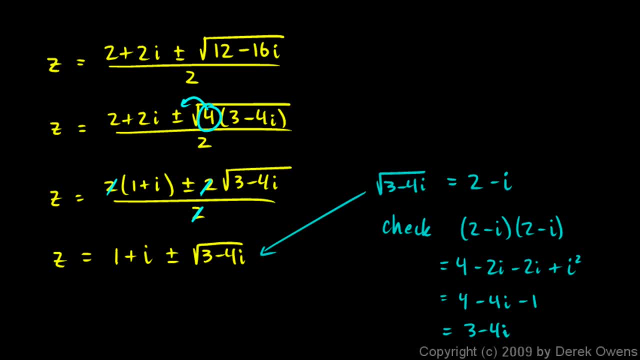 So 2 minus i squared is in fact 3 minus 4i. So the square root of 3 minus 4i is 2 minus i. So that means z is equal to 1 plus i plus or minus 2 minus i. 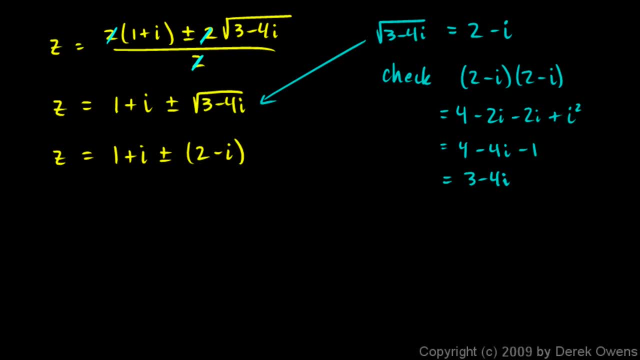 OK, let me scroll down a little bit more. So let's just work out: each of those z is going to be 1 plus i plus 2 minus i, Or it's going to be 1 plus i minus 2 minus i. 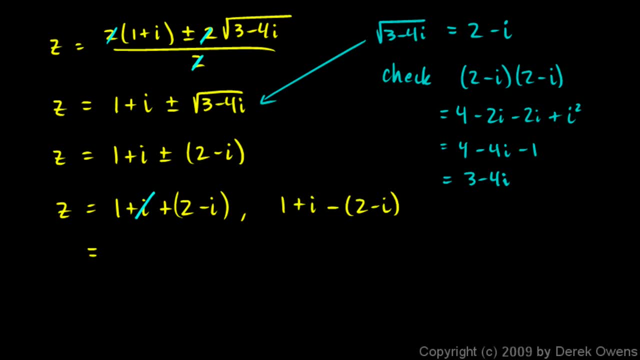 So 1 plus i plus 2 minus i. You can see this plus i and the minus i canceling, And we're just left with 3.. That's one of our answers. And then over here: 1 plus i, minus, 2 minus i. 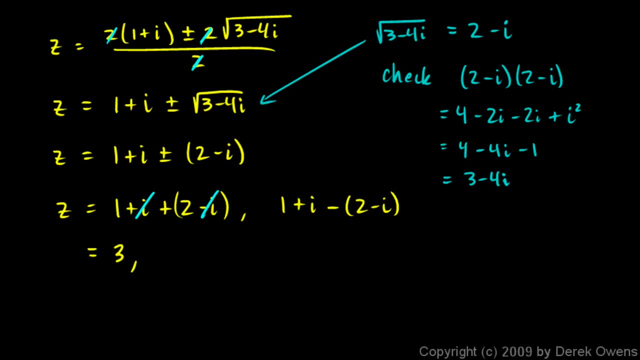 This minus right here distributes right there, So that's really a plus i So just tracing this through, this is 1 plus i minus 2 plus i. We end up with negative 1 plus 2i, So again it's a quadratic. 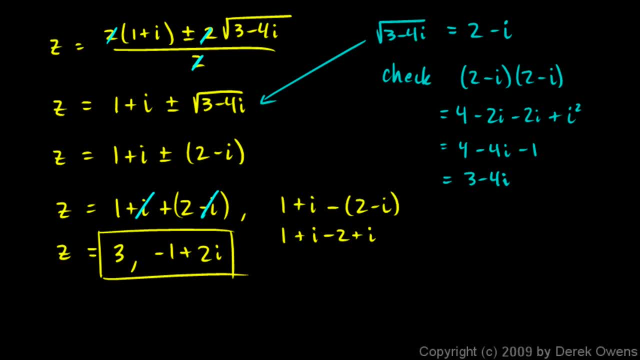 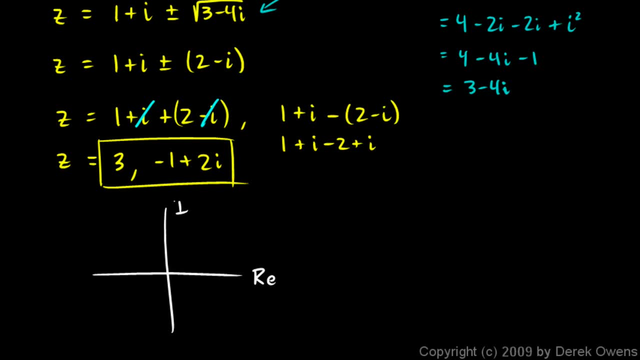 We typically have two solutions to a quadratic. And there they are. We can visualize where these are if we just sketch a square root. We can visualize where these are if we just sketch a complex plane real quick. Here's our real axis And here's our imaginary axis. 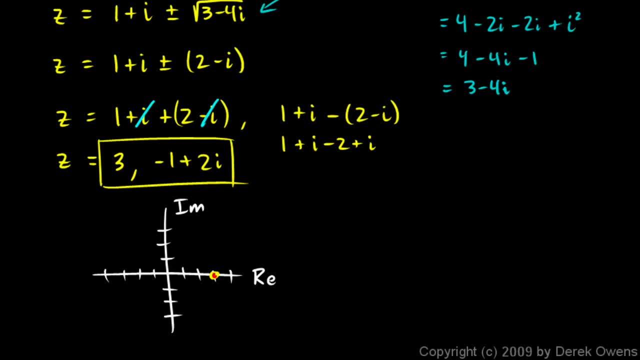 The number 3 is right there, And then the number negative, 1 plus 2i, is right there. So two solutions, And there they are, And I'll come back in the next video and elaborate a little bit on getting from here to here.